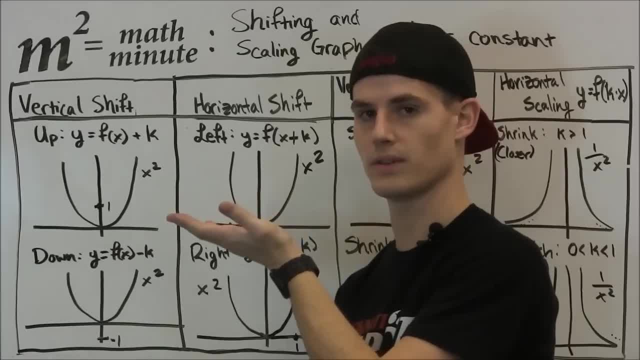 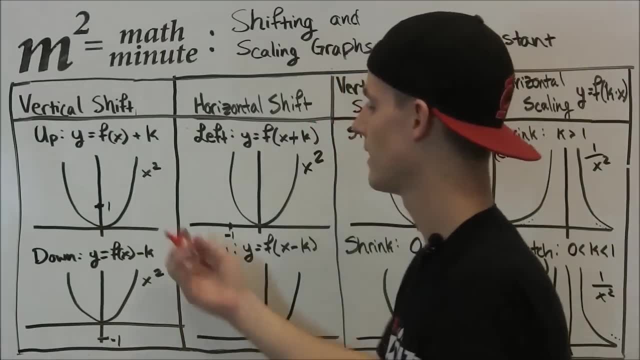 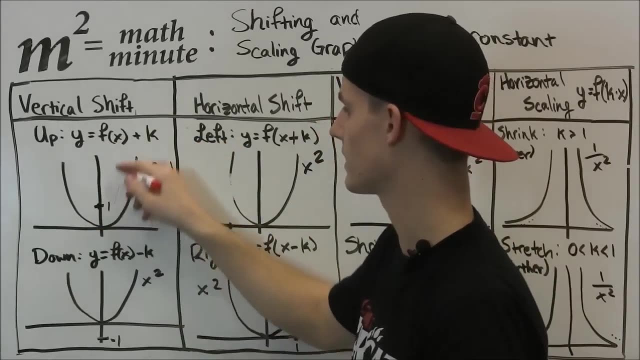 some value k to it. we're going to shift it up that number of units. So, as you see, with all these I have x squared drawn. That's the easiest graph to understand. So what we're going to do is if we were to say x squared plus one, this is going to shift this x squared. 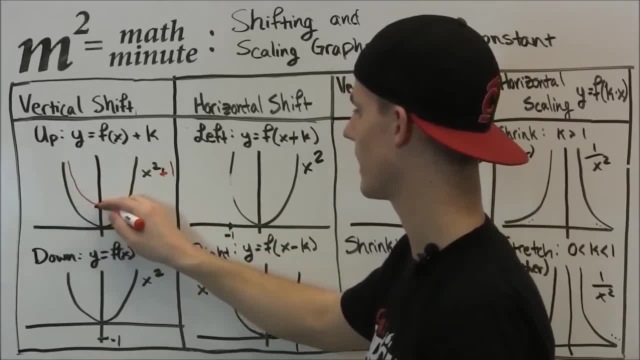 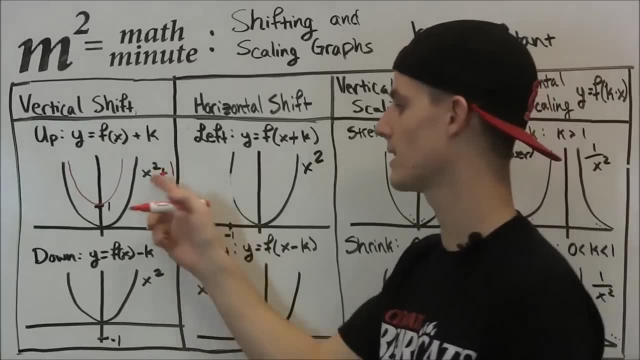 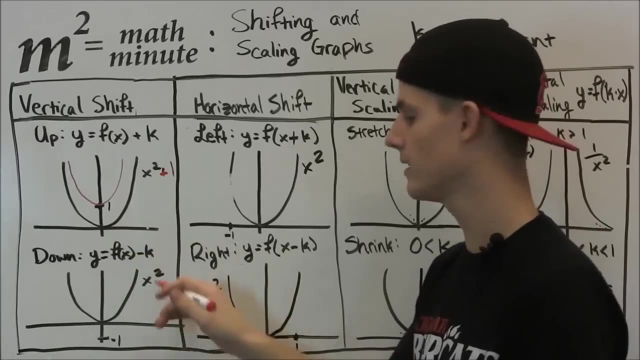 graph Up one unit. So this is then what we're going to have: The same graph, identical graph, but up one unit. Now, if you can kind of guess, if we were to subtract that k value, we would probably shift it down. So now, if we have a function minus some constant k, we're going 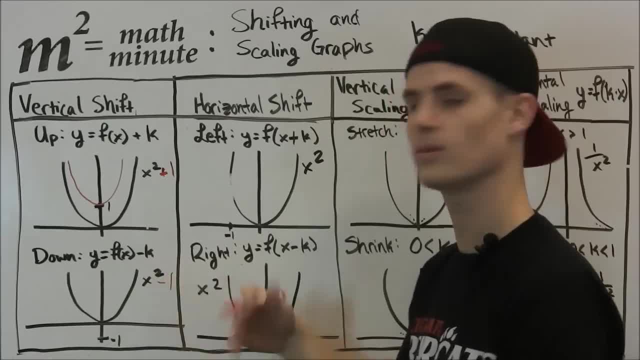 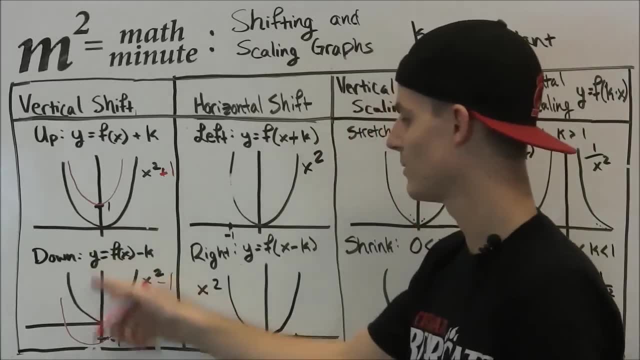 to shift it down k units. So in this case we're going to have minus one. So once again, we're going to draw the exact same graph, x, squared as good as we can, and we're just going to draw it down one unit. 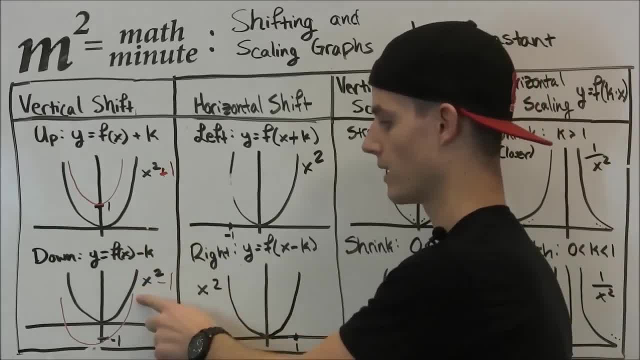 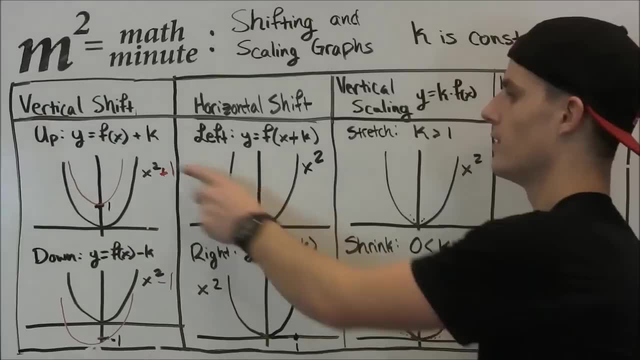 So this would be the graph x squared minus one. It's the graph of x squared just down one unit. Now we're going to talk about horizontal shifts. This gets a little bit more confusing. This was outside the function, so after we already did the problem, we had our answer. 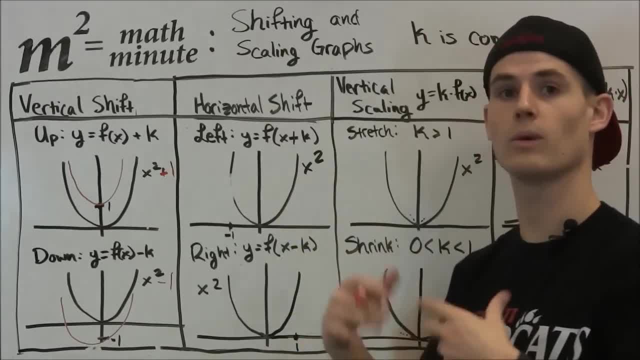 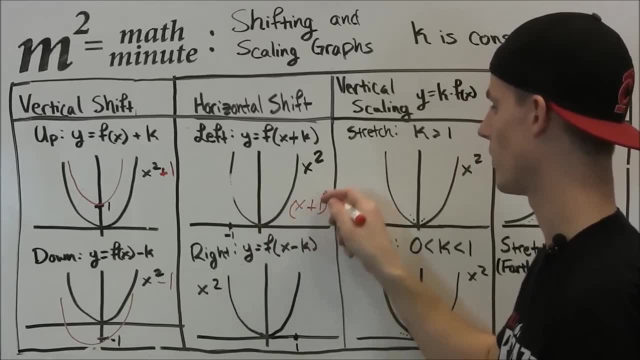 we added the value to it. This we're going to add while we're inside the function. So in this case this would be like x plus one, the whole thing squared. So before we're actually finding the answer, we're adding it to the x value. So this is going to be x plus one. 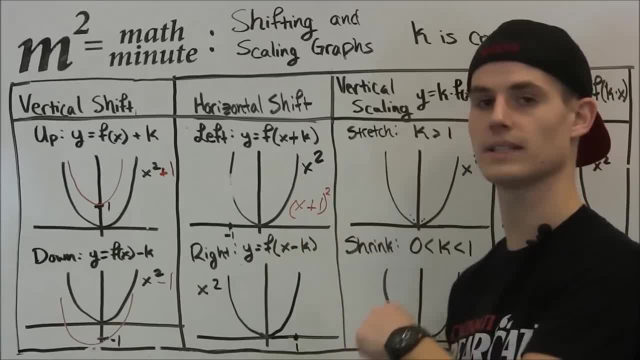 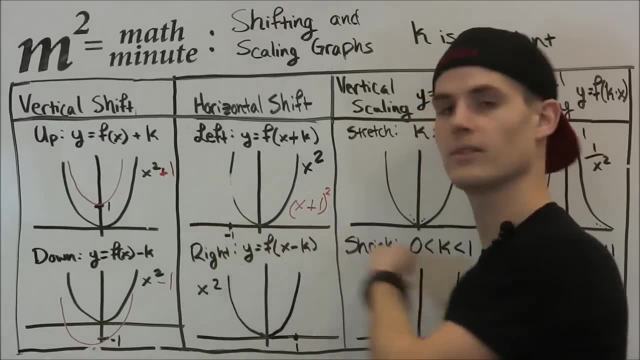 So what this does is this is going to shift it left one unit, and this is when we add. This is kind of confusing. Sometimes you want to say we're adding, we're going to go down to the right when we go down x values, but actually, with a horizontal shift, we shift. 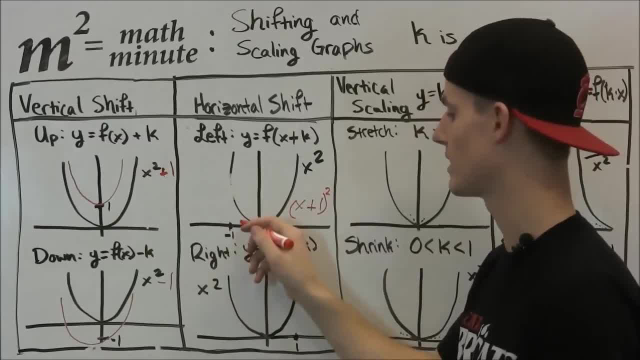 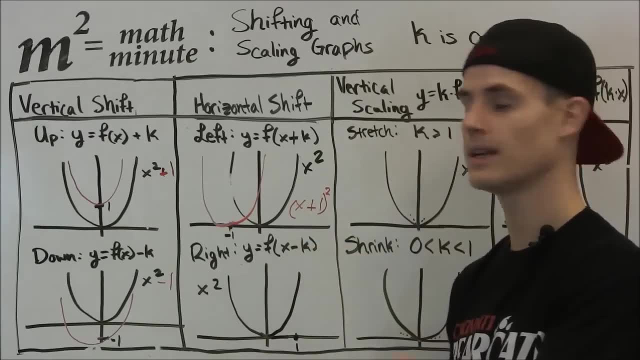 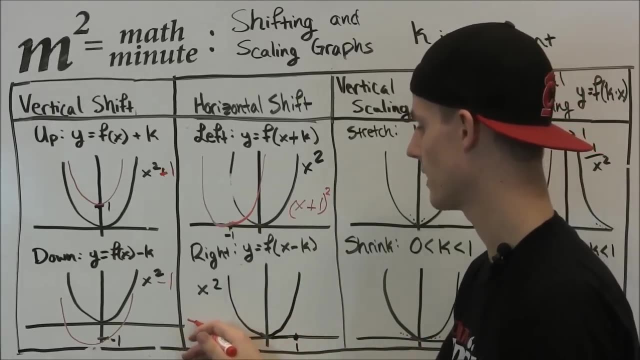 left if we add on the inside of a function. So, as you can imagine, it's going to be the same graph just shifted to the left, one unit Now, kind of similar to vertical shift. we're going to do the opposite when we subtract. So if we're talking about a function x minus, 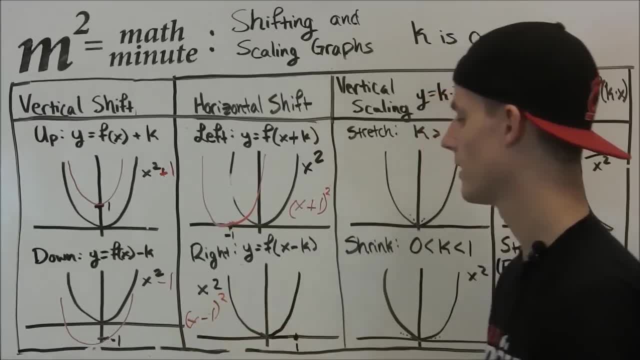 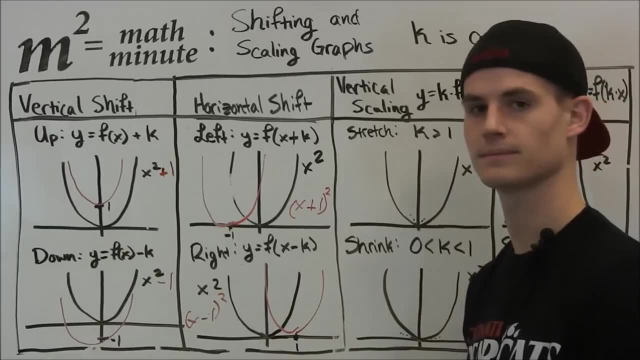 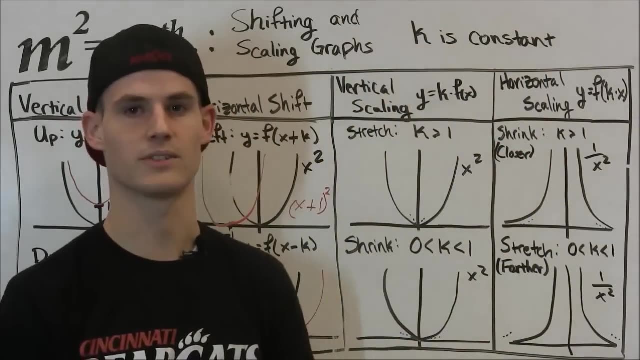 one squared, we're going to shift it to the right one unit, Just like that Same graph as we had before, x squared, just shifted to the right one unit. Now this is where things get a little confusing. We're going to talk about vertical scaling. so what we're going tackling all the verticals with is: we're going to work it out very here. so when we clerk on the front, next we're going to 집 on the bottom, afect. 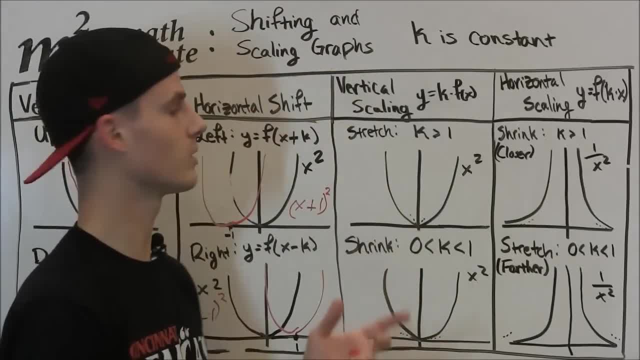 we say we're trickling across theiation, but we automatically get two st końung the job, and then we Mosこれで. What we do now is when we multiply by a value, we're going to change it in a different way. 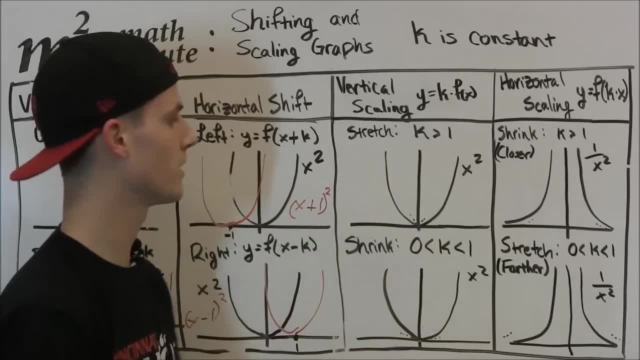 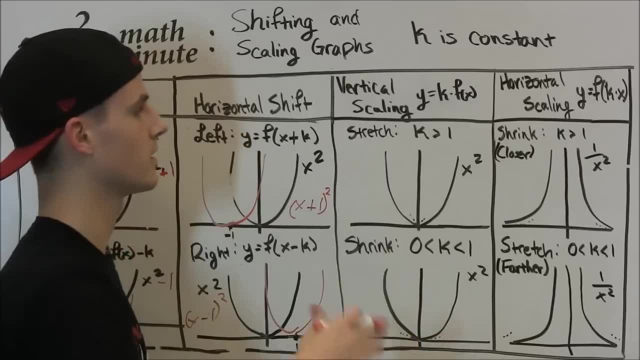 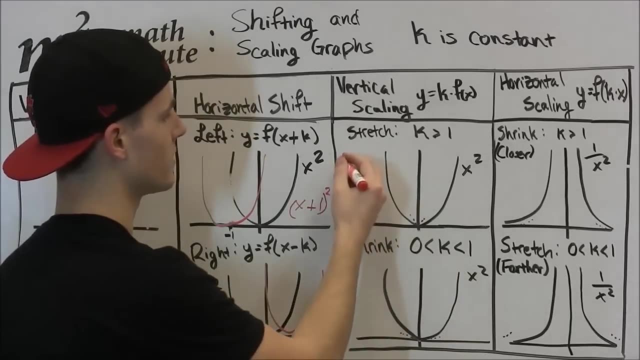 We're going to call it vertical stretch or vertical shrink. So in this case, if we have y equals a constant times f of x outside the function, we're going to stretch it if k is greater than 1.. So let me draw an example and we'll talk about it. 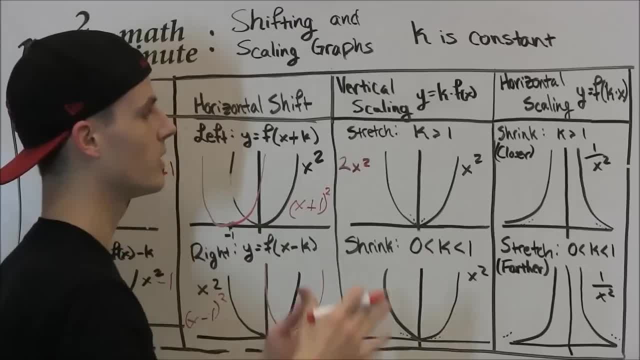 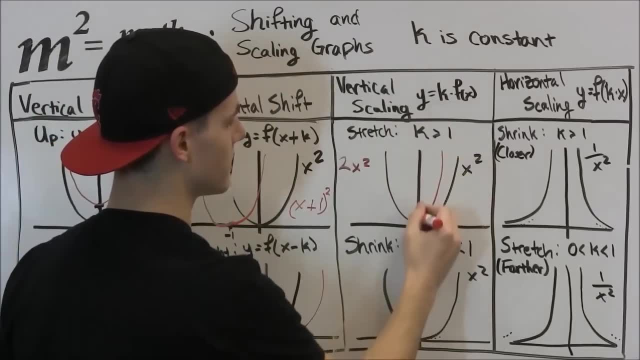 So if we had 2 times x squared, we're going to stretch this vertically, So we're going to take the function, we're going to go like this, We're going to pull it up like that. So this is what 2x squared is going to look like. 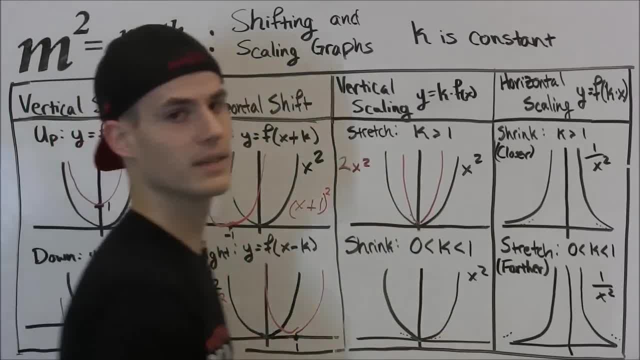 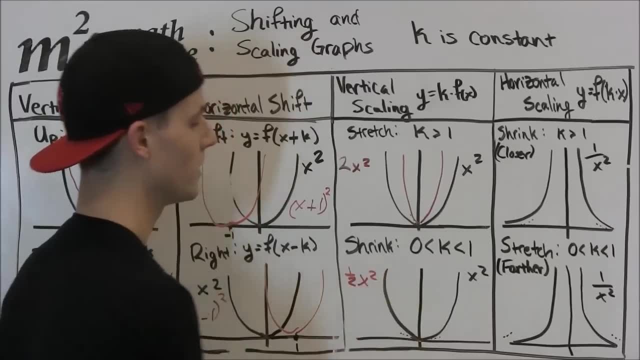 Now, if we had, x was between 0 and 1, that means that it's a fraction, That means it can't be 0, it can't be 1.. So let's talk about 1 half times x squared. So what this is, this is shrink. 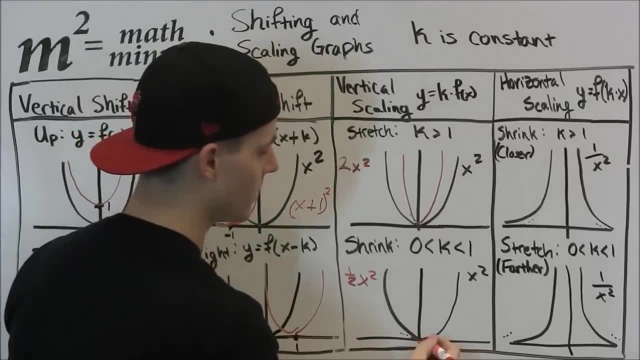 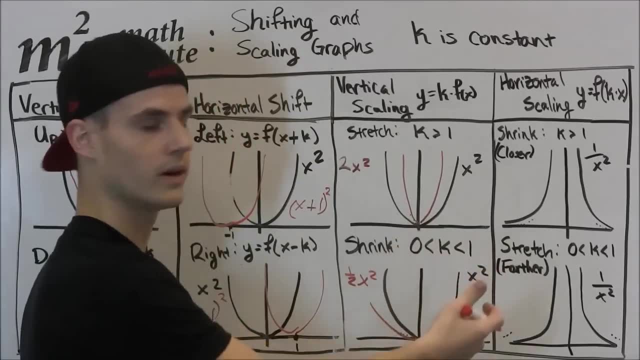 We're going to smash it together. So if we had something and we smashed it together, it's going to go outwards like this: So this would be the graph: 1 half times x squared, So anything that's between 0 and 1.. 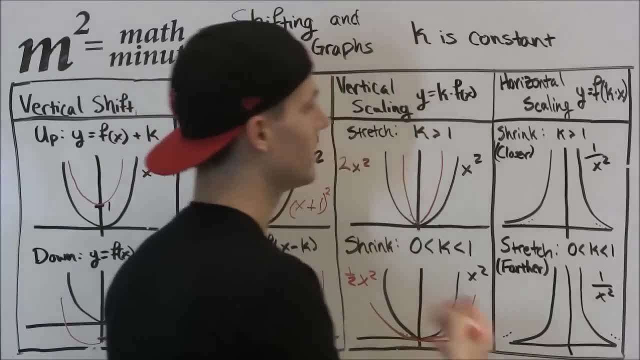 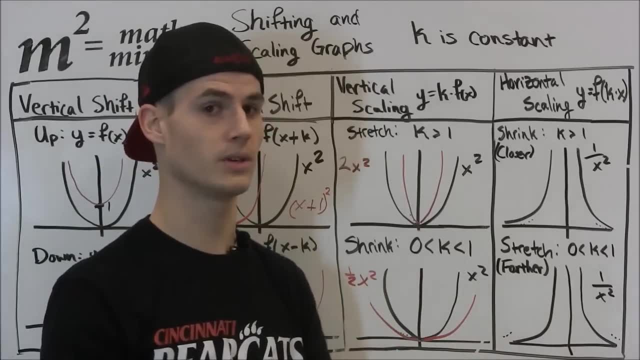 When multiplying by this function, we're going to smash it. Now this is where things get really confusing. Horizontal scaling There isn't really. it's kind of explained properly in the book, but this is where certain examples it's the same as vertical scaling. sometimes it's not. 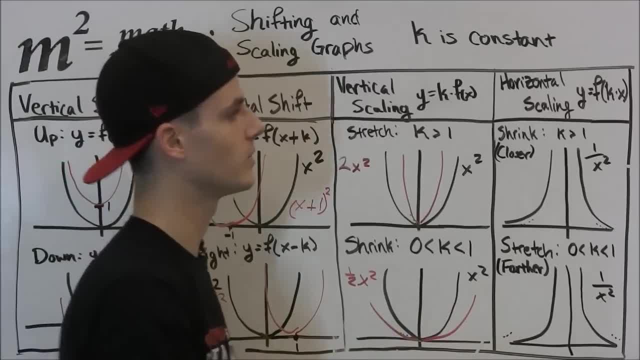 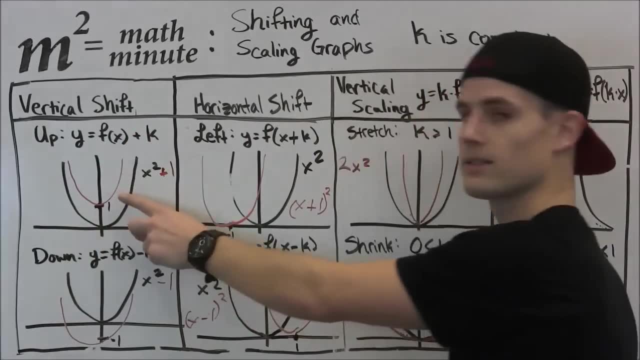 So this is an example of 1 over x squared. This is a good example of when this will actually apply If k is greater than 1, and we multiply this on the inside of the function, Just like here we had on the outside and then the inside. 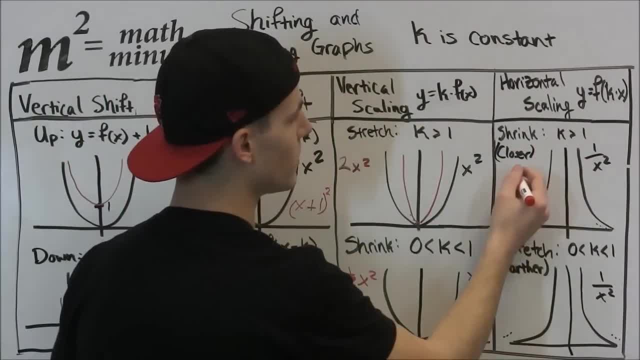 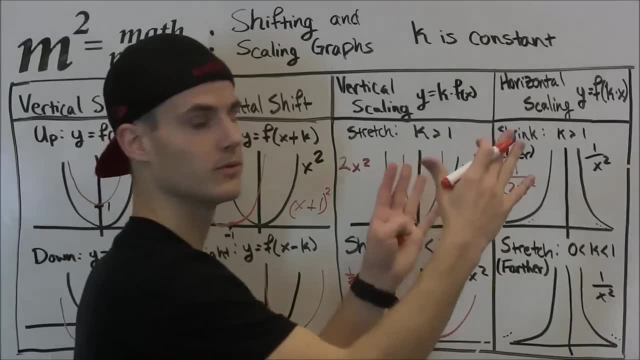 This was the outside, This was the inside, This was the outside And this is going to be the inside. So if we multiply this inside by 2, what's going to happen is this is going to move towards the x axis. So it's going to be the same graph, but just closer to the x axis. 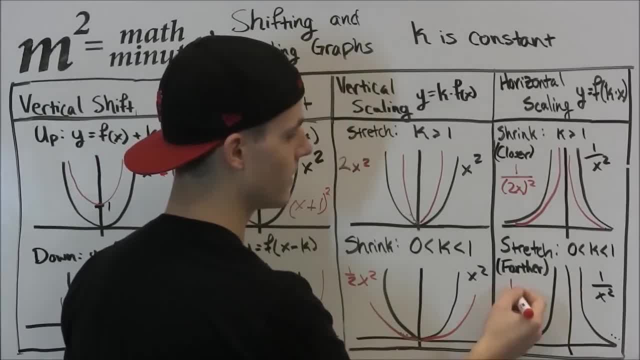 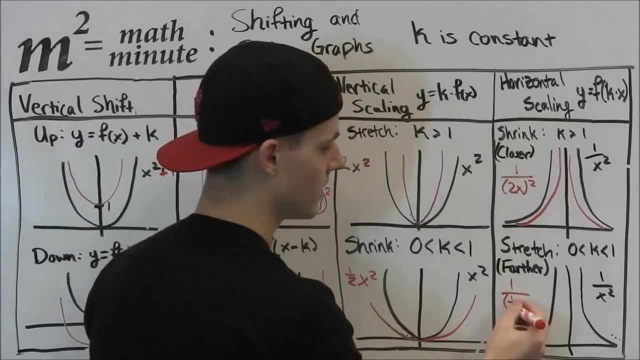 So now, if you can imagine, what's going to happen is if we multiplied the inside by something that's between 0 and 1. Well, if this moved it closer to the x axis, if we multiply the inside by 1 half.